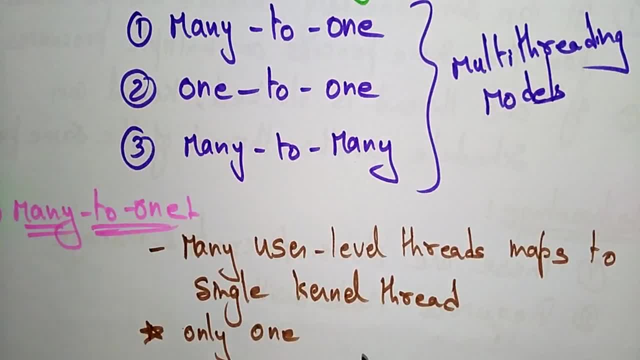 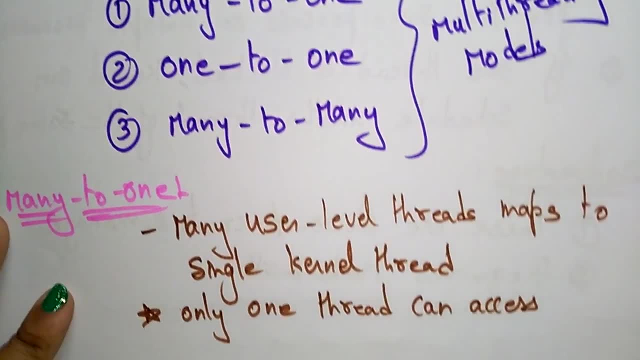 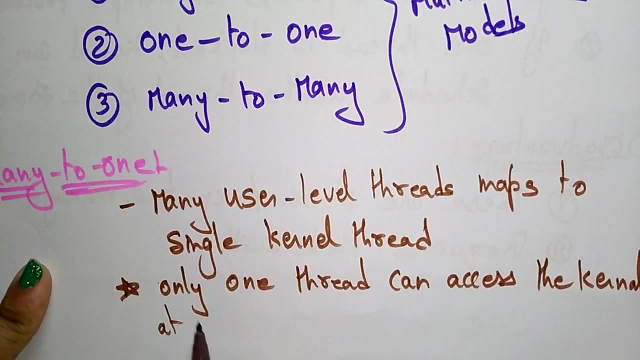 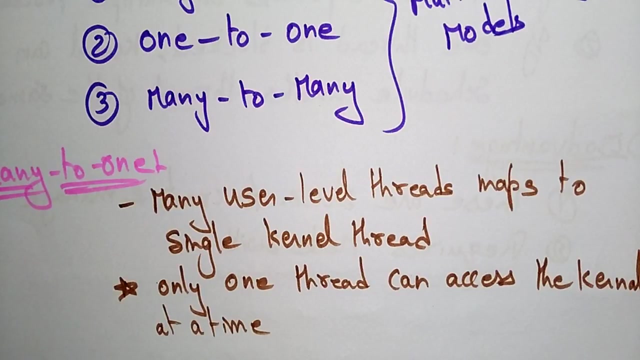 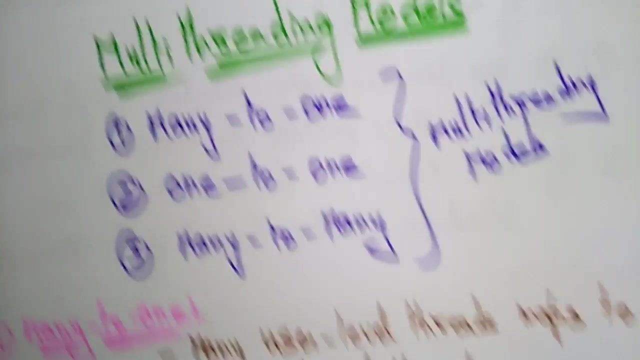 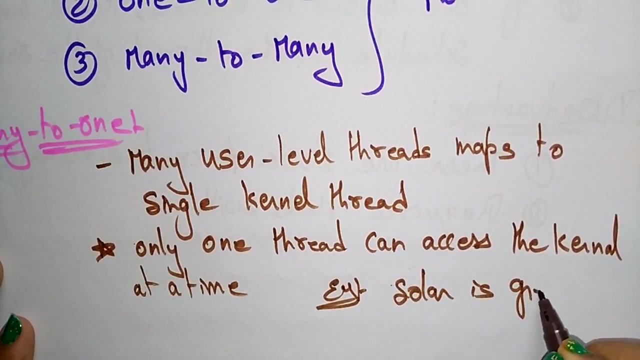 many user level threads are there, But it can accept only one thread can access access the kernel at a time. So multiple threading are unable to run in parallel on multi-processor, So that is one disadvantage in using the many-to-one concept. So let us the examples for this many-to-one or examples. or solar: Solar is green thread. 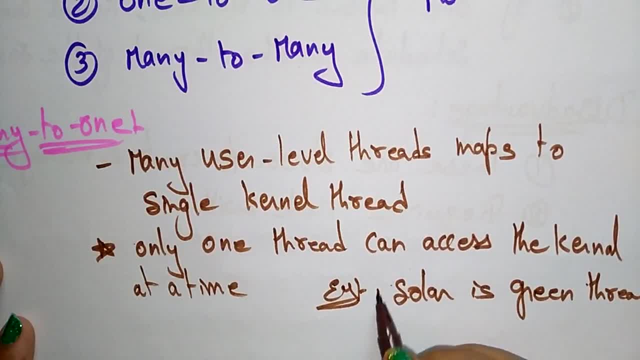 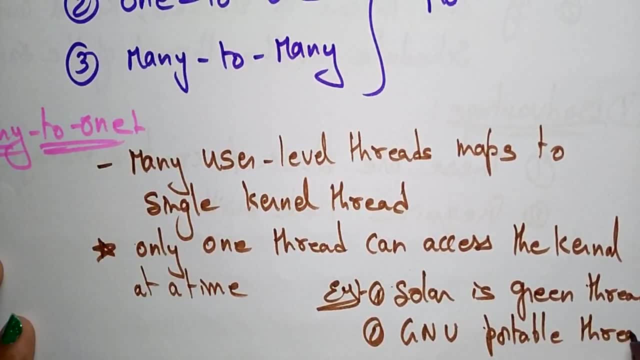 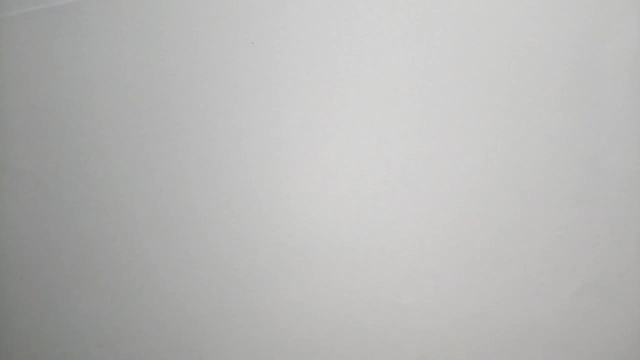